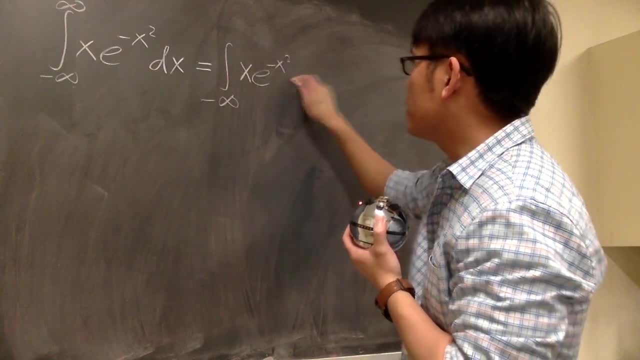 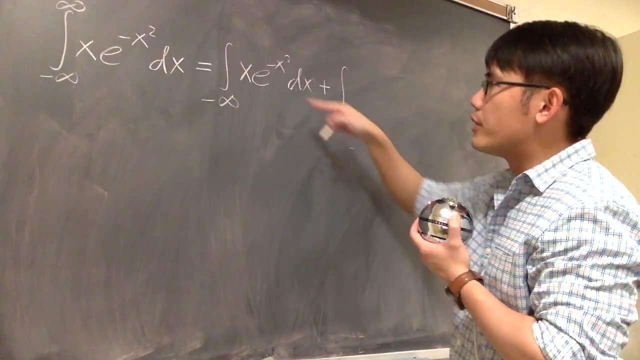 The inside will stay the same x times e to the negative x squared dx, And then we will combine with the second integral And then for the starting number right here, this number has to be the same as that number of your choice, And then the top right here will be the infinity. 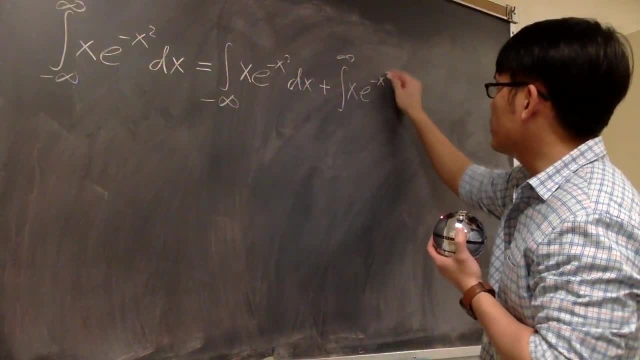 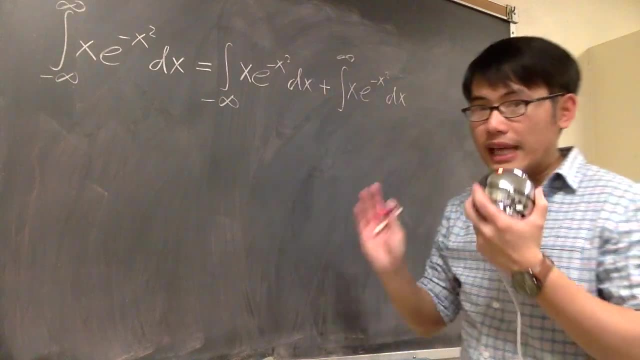 And of course, the inside will be x times e to the negative x squared dx. And now the question is: what should I pick for this number and that number? As long as it's finite, as long as they are the same, It's okay. 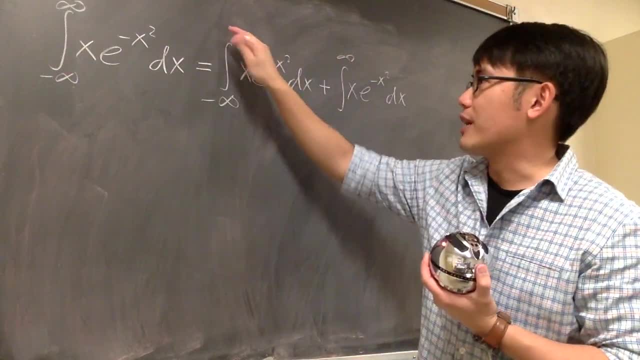 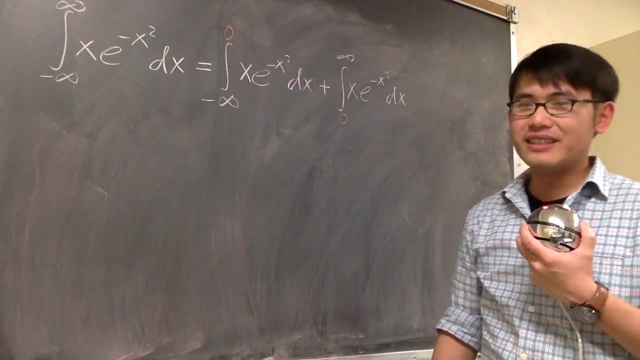 You can put one right here, one right here, that's good. You can put a five right here, five right here, But then you cannot beat the zero here. the zero here. Perhaps that's the easiest. So that's why I chose the zero and zero. 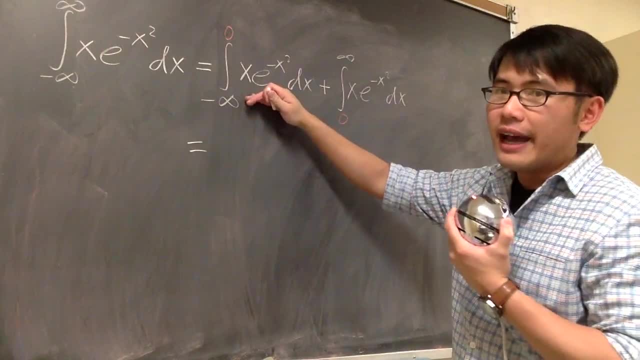 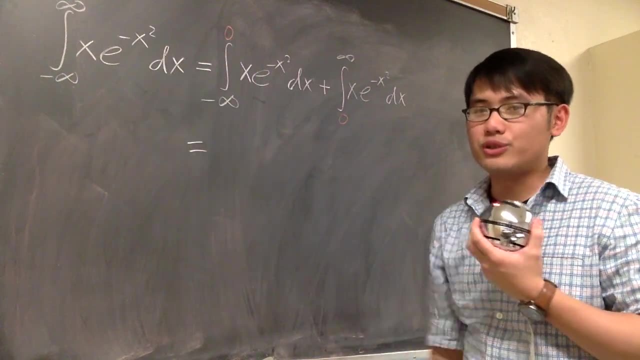 Okay, so for the rest of this, I'm going to integrate this guy and then believe in my limits, work it out. If I get a finite answer, that will be the answer. If I don't, then that means the integral diverges. 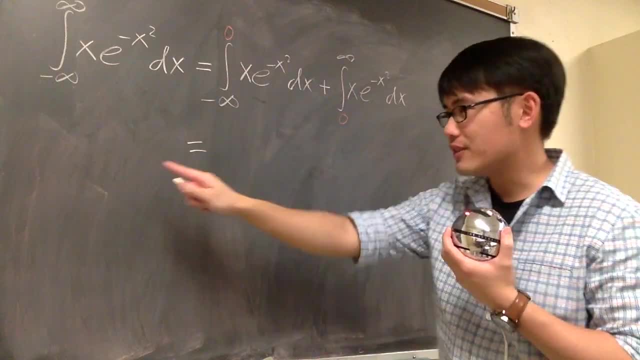 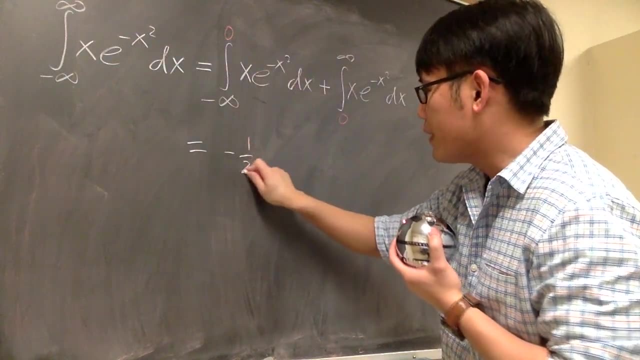 So we will have to get the anti-derivative for this guy. So you can watch this video right here and then you can see how we can do the anti-derivative. But I will tell you the answer for this is going to be negative. one half e to the negative x squared for the anti-derivative portion. 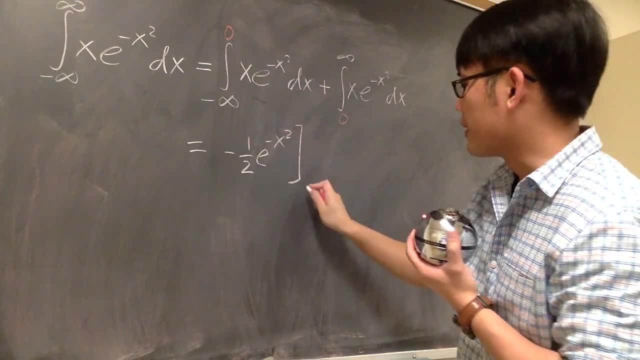 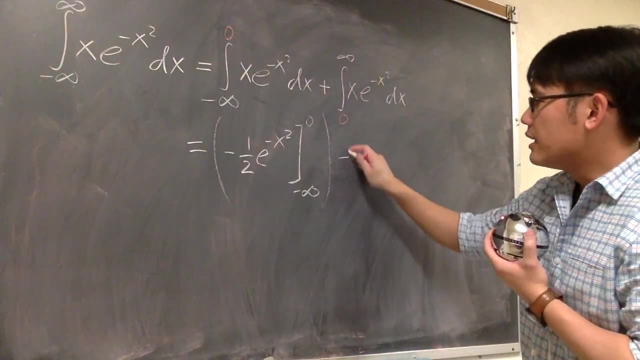 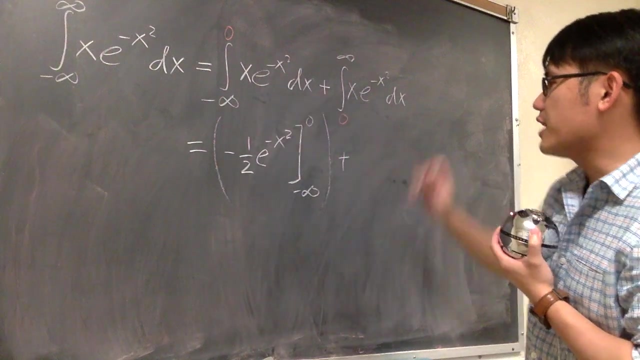 And then, for the first part we're going to focus on from negative infinity to zero. So this is the first part to focus, And then the second part. once again, I have to do the anti-derivative, And then it's going to be the same anti-derivative, because the insides are the same. 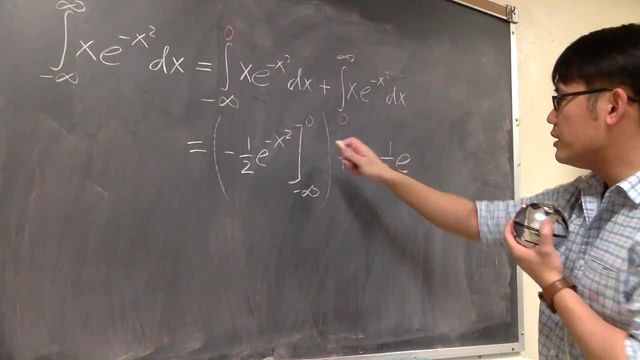 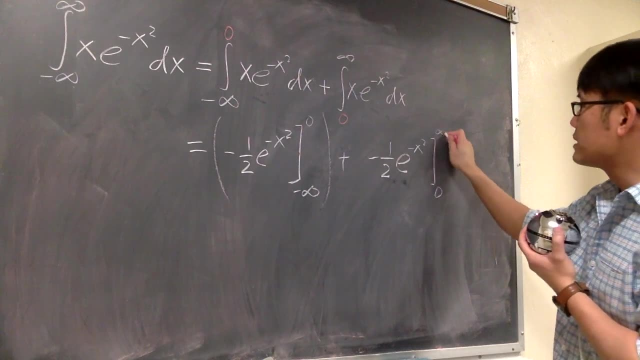 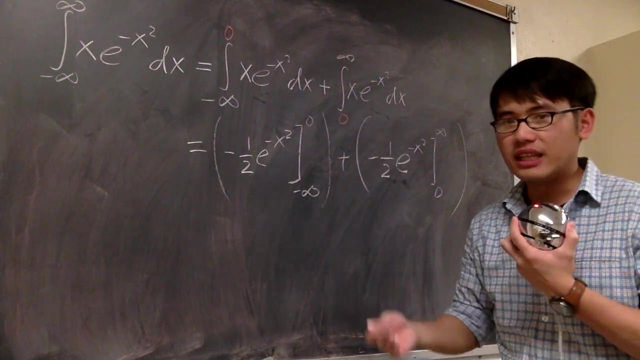 We will have negative one over two, e to the negative x squared, But then in this part we are going to go from zero to positive infinity And hopefully I can get a finite answer from both of these. If not, then that means this integral diverges. 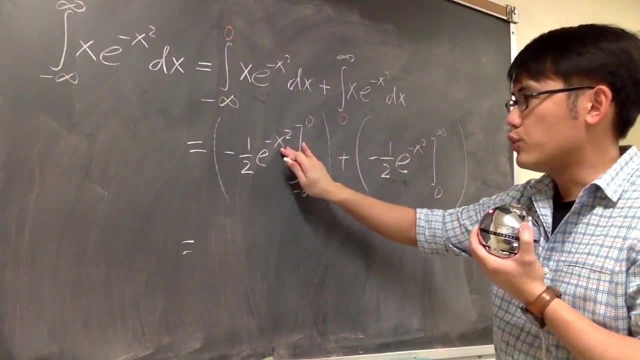 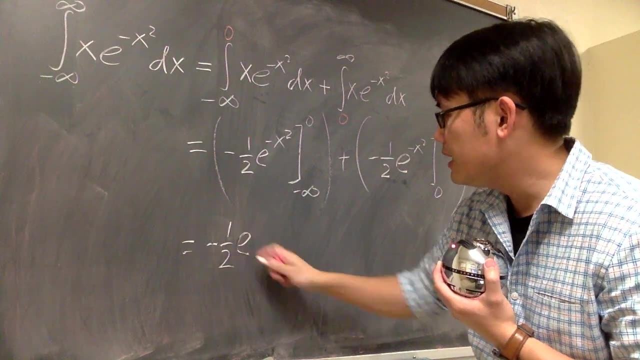 So for the first part, right here, I'm going to plug in zero into x, first Subtract, right? So we are going to have negative one over two, e to the negative, zero to the second power. But then let me just show you. 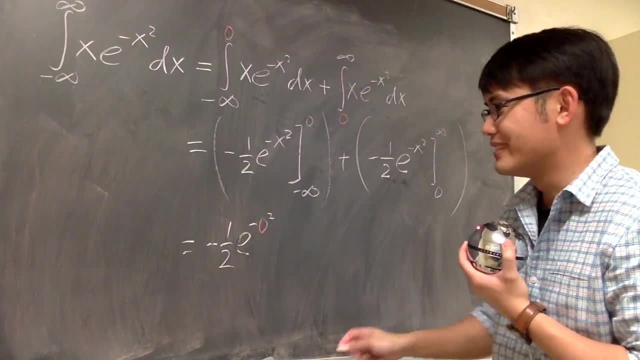 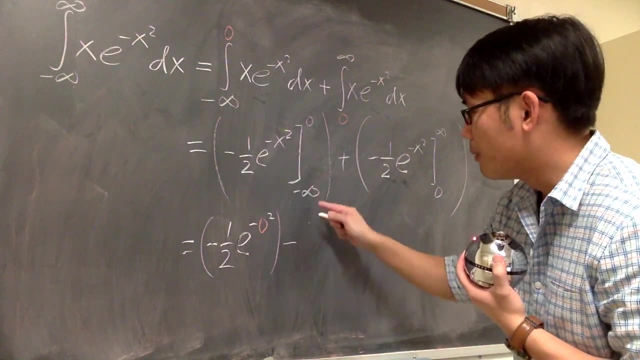 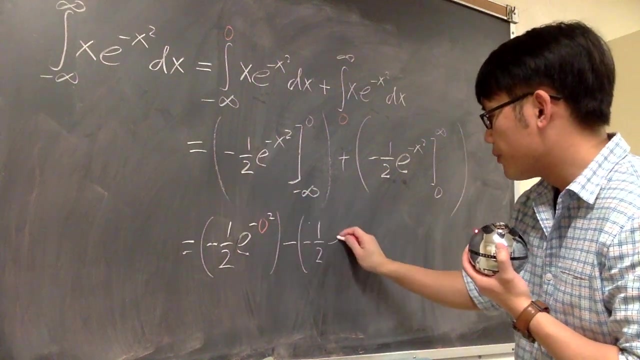 Here I have my zero and then here I have my square. So this is the first part. After I plug in zero into x And then I will subtract, Plugging negative infinity into this x, we have negative one, half e to the negative x squared. 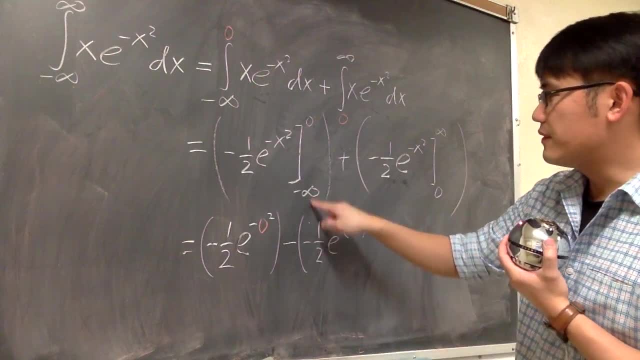 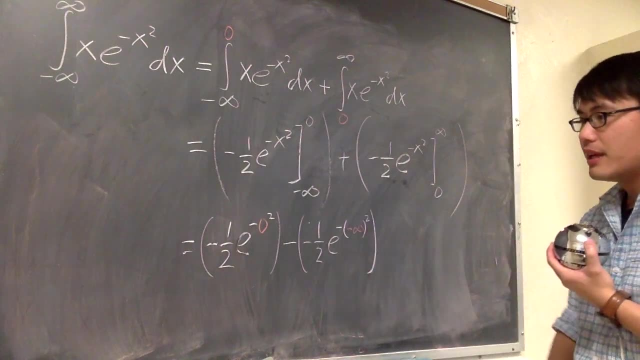 Negative, then we open the parentheses and then plug in negative infinity into x, But then we still have this part being squared. Okay, So that's the first part from here, And then I have to add this part. And what do I do? 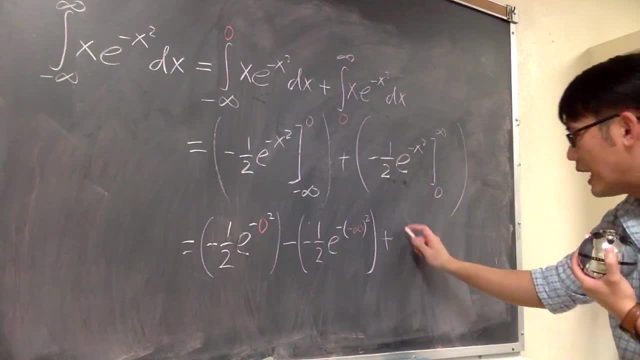 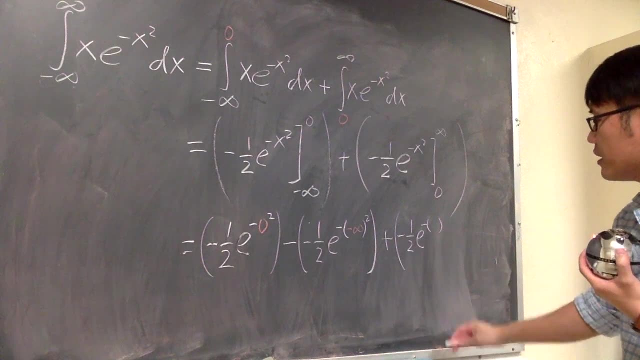 Well, I plug in infinity into x first, So I will have negative one, half e to the negative. Then we open the parentheses, We have the negative here, And instead of this we have positive infinity, And then we have to do this square. 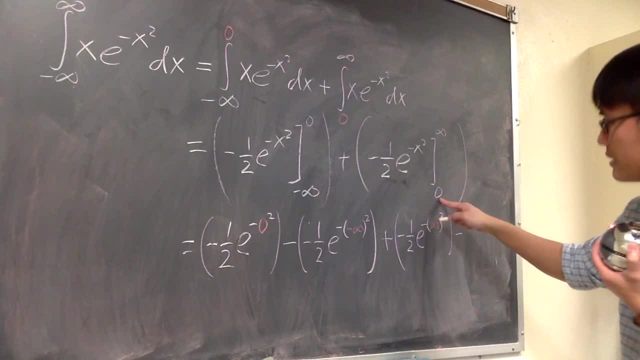 And then we will subtract And you plug in zero in here And this is going to be negative one half And we have e to the negative, zero squared. So let me just do this for you guys: Zero squared. So that's the setup. 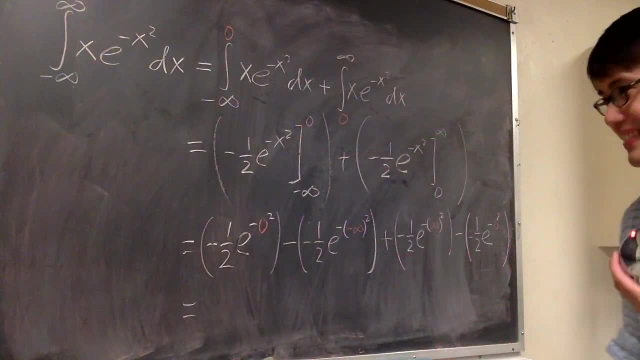 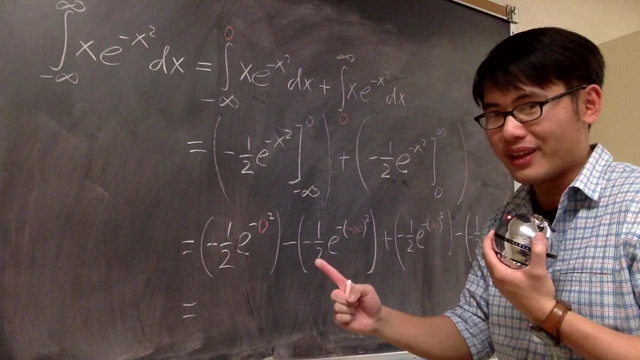 Not too easy, Not too hard. Everyone can handle this Right, All right. So this is going to be what? This is good, because this is e to the zero, which is just going to be one Negative zero, which is the same as zero. 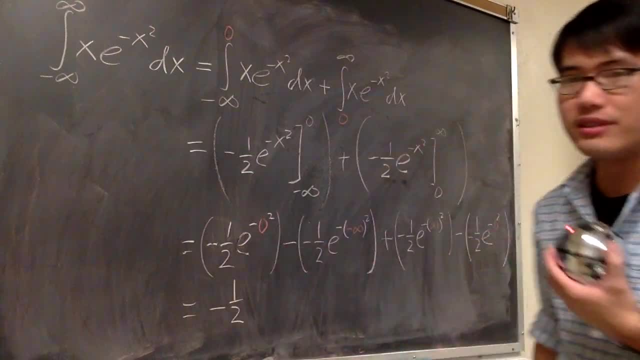 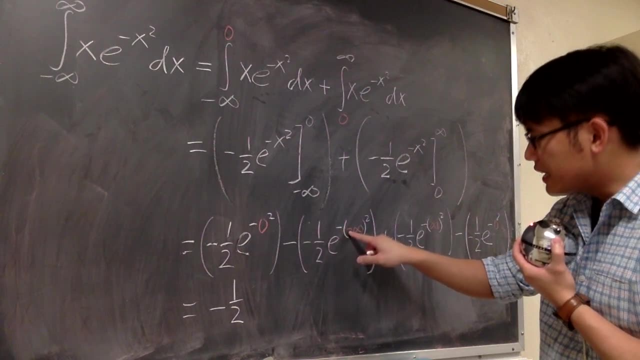 So we have negative one half for this parentheses. And what's this? Check this out. This is e to the negative. But then you look at this: This is negative infinity to the infinity, which is negative infinity. Right, This is infinity. 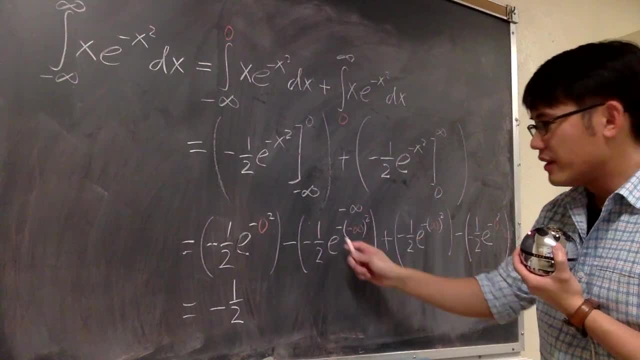 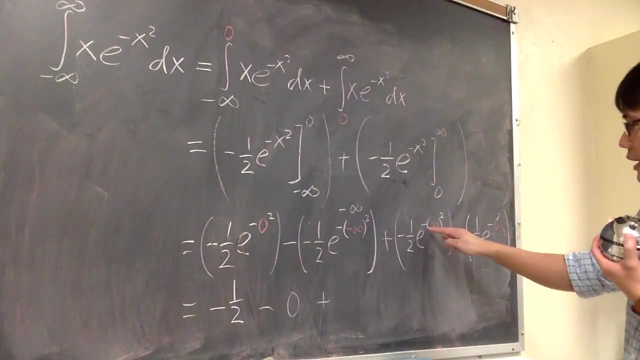 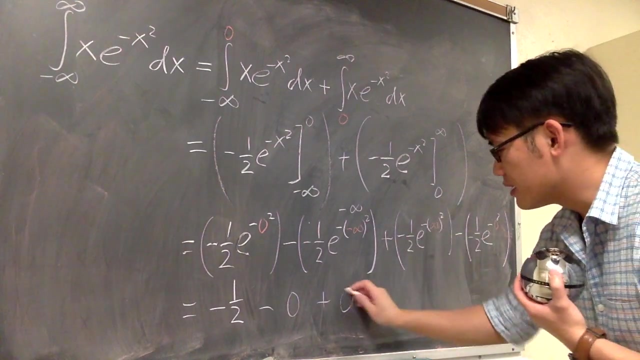 But then you have this negative e to the negative infinity. This part is going to be zero Minus zero Plus. how about this one? Well, infinity to a second power is infinity. e to the negative infinity is zero And negative one half times zero. it's once again zero. 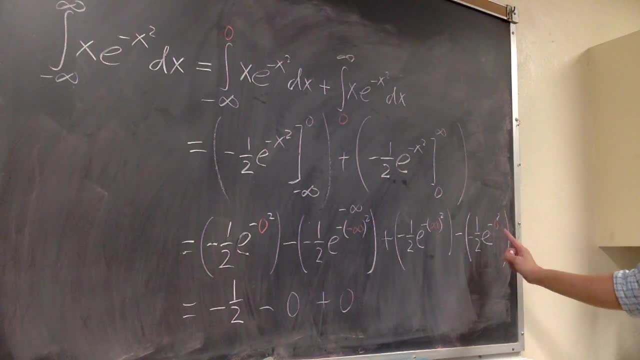 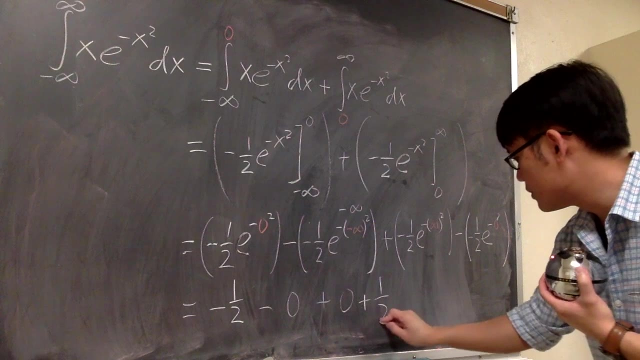 And the last part is: what e to the zero power, which is one, But this is negative one half. We subtract negative one half, So we plus the one half, Right. And what does this mean? This is negative one half.